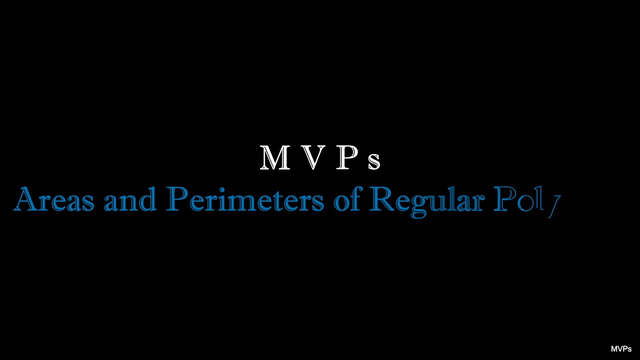 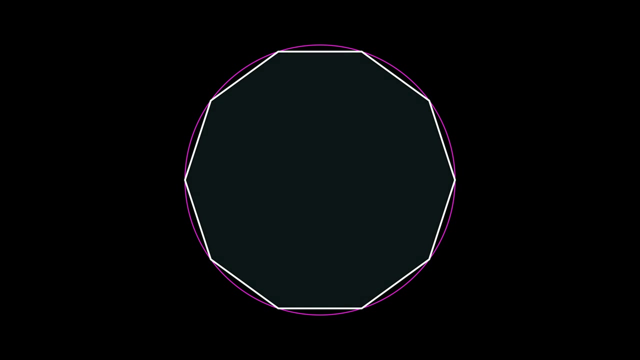 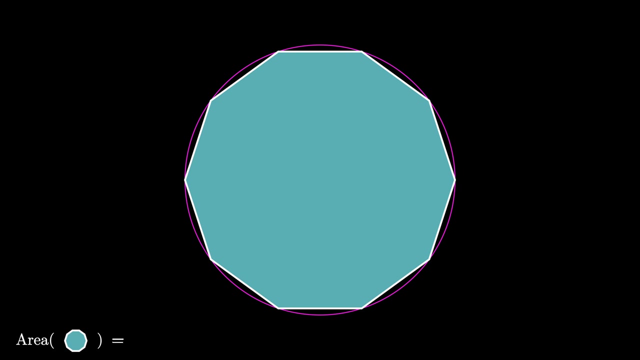 Start with a circle of radius r and then draw an inscribed regular 2-ngon like this. Let's figure out the area of this regular 2-ngon. To do that, we can decompose the polygon into triangles. The radius of the circle is r and there are 2n copies of this triangle. 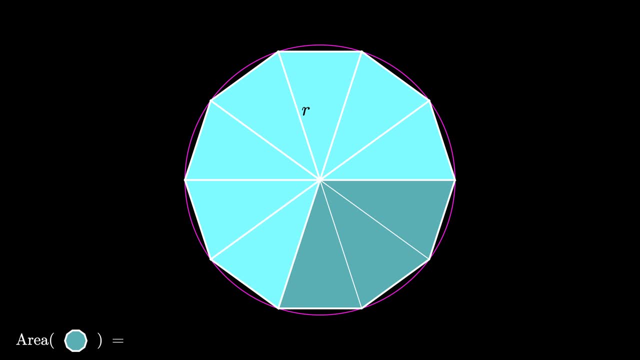 that can be used to build the regular 2-ngon. So the area of the regular 2-ngon is 2n times the area of one of these triangles. Now let's draw the inscribed regular n-gon like this and suppose that this n-gon has: 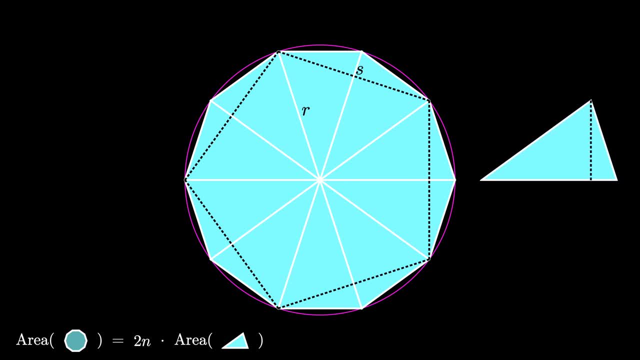 a side length of s, Then the triangle that we're interested in has a height of length s over 2 and a base of length r. Therefore, the area of the regular 2-ngon is 2n times 1, half times r times s. 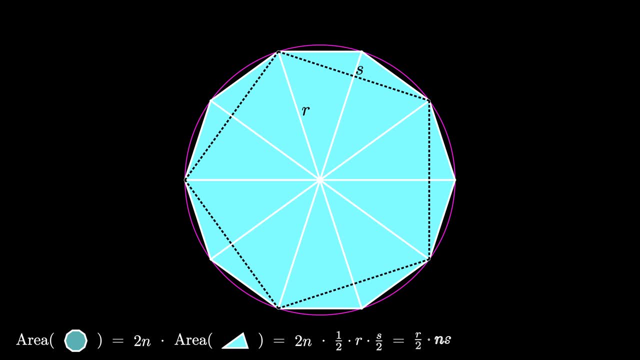 over 2.. But this simplifies to r over 2 times ns and ns is the perimeter of the regular n-gon inscribed in the circle. But this means that we have shown that the area of the regular 2-ngon inscribed in a 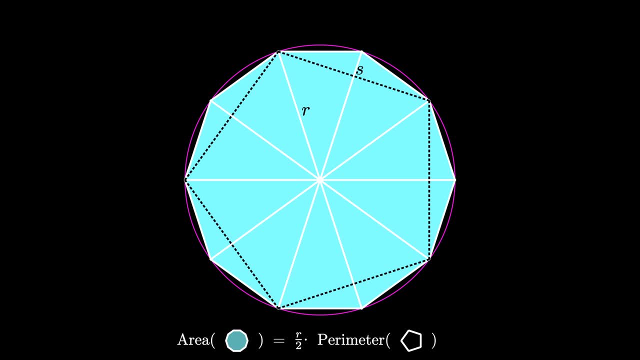 circle of radius r is equal to r, over 2 times the perimeter of the regular 2-ngon inscribed in the circle. But that's not all we can say, Because both the 2-ngon and the n-gon approach the circle as we. let n go to infinity, we 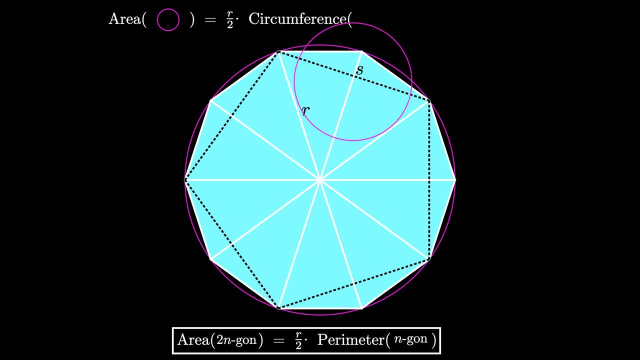 get the result that the area of the circle is equal to r over 2 multiplied by the circumference of the circle. If we remember that the circumference of the circle is 2 pi r, then we see that we've found a formula for the area of a circle of radius r to be pi times r squared. 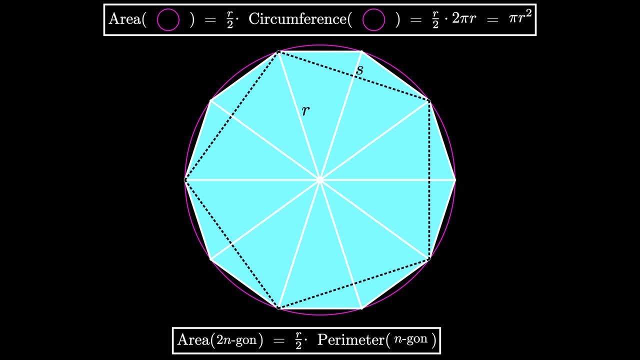 We actually know that if we search this simple formula, references to r are not momentarily valid and that we put them in proper order. every time we check the formula we should find the answer in the dot to every time. Thanks for reading to last year's. если you enjoyed this, it very much. 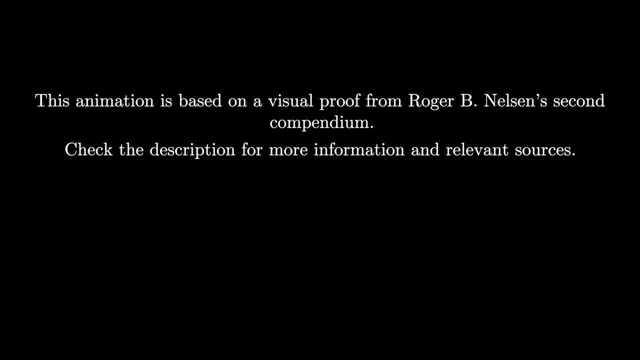 It's good that you like it. Thanks for checking this out and please leave a comment with your favorite comment If there are any noting other than thank you. how I unintentionally said something there, let it go in a roll so that I don't spend more time with you in the next video and I will see you in the next one. I'm é Donald shining. you all dears.